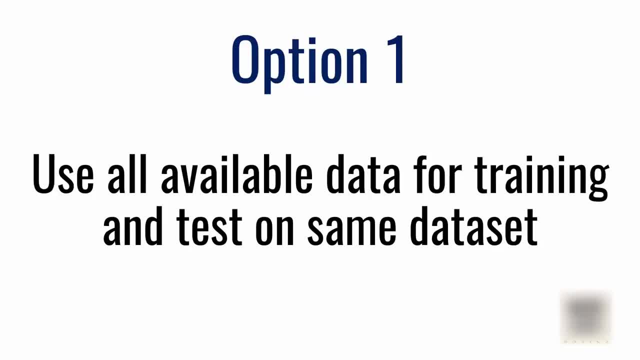 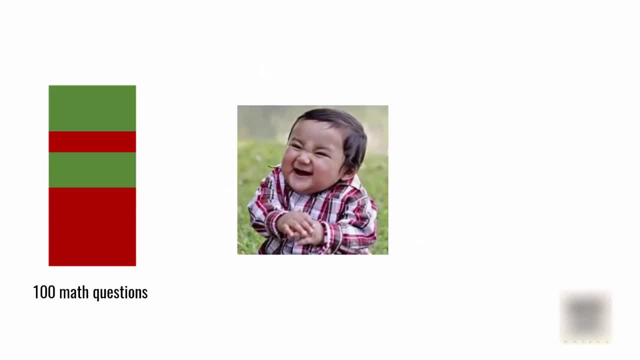 to train the model And then you use the same exit samples to test the model. This, in real life, can be compared to an example of preparing this cute kid for a mathematic test. So let's say you have 100 mathematical questions. you train this kid for those questions. 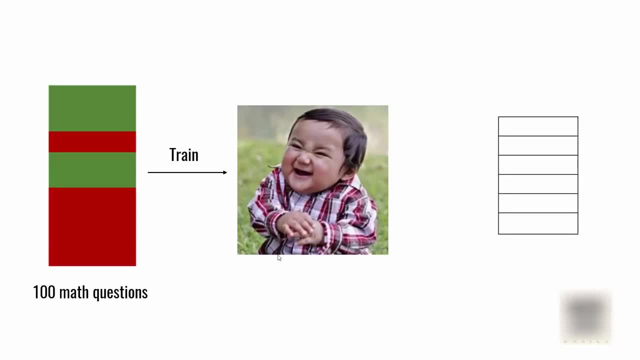 And then when he goes for the exam, you ask the exact same questions, okay, and then you try to measure his mathematical skills based on the score. Now, this is not a very good way of measuring someone's math skills, because he has all the 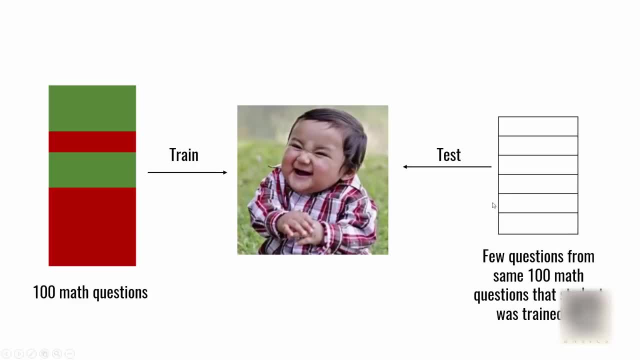 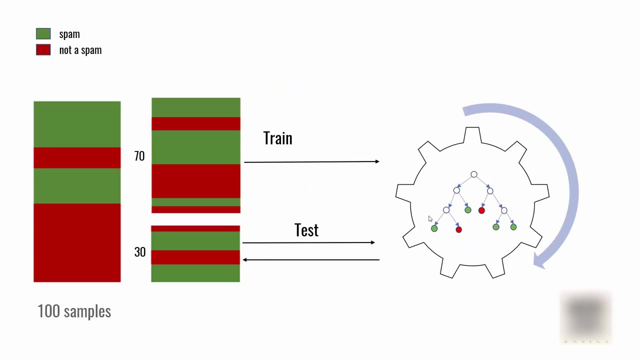 seen those questions before. Alright, so what if he gets like 100 out of 100, there's no point, he has already seen them. So then the second option we have is we split the samples that we have available into training and taste data sets. So for example, here I will, I will out of 100,. 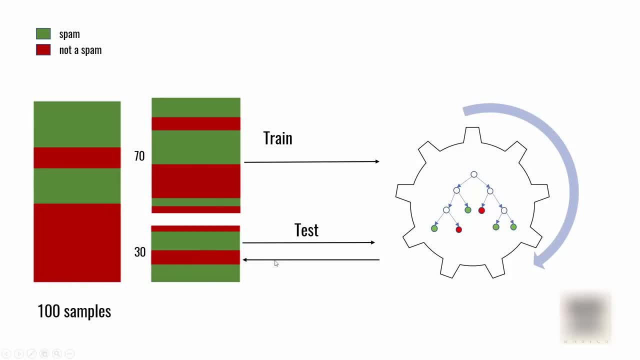 I will use 74 training and 34 testing. Okay, And we have been using this train test split method in all of our supervised learning model tutorials, And you will see that we have used train test split method in, I think, majority of our tutorials. So that's what. 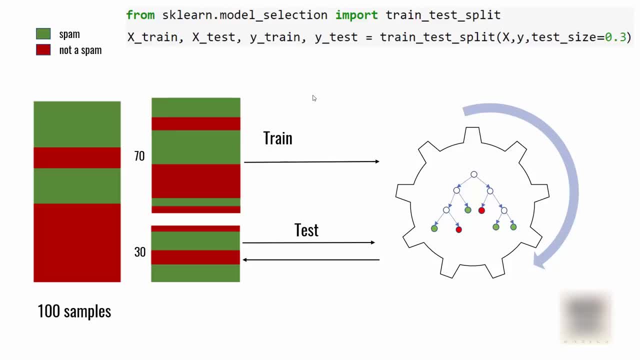 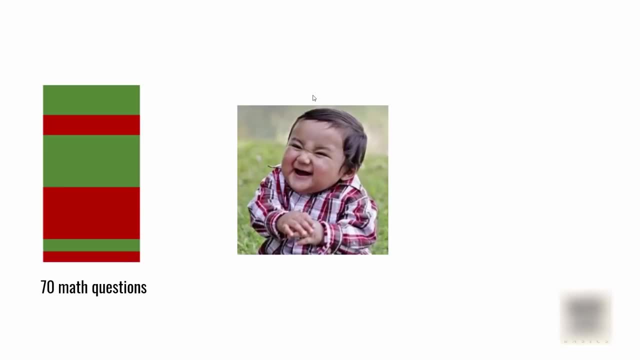 this technique is. So, again going back to our student example, you give this person 70 math questions for preparation and the remaining 30 you will reserve for the test. So that way, when he goes for the test, he has not seen these 30 questions, which is good. that way you can measure. 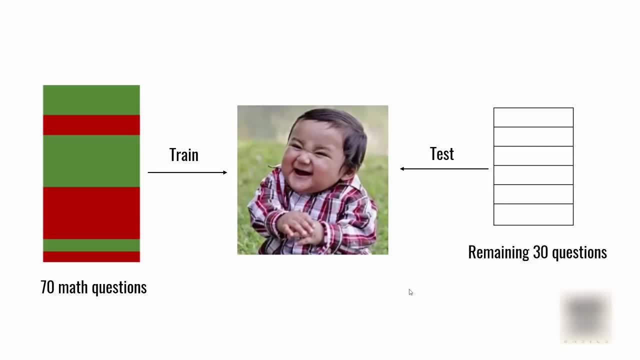 the skills in a good way. But there is one problem with this approach also. let's say 70 math question that you give this person. let's say they were all algebra and now remaining 30 questions are from calculus. So now those questions he has not seen before or he doesn't have knowledge on that. 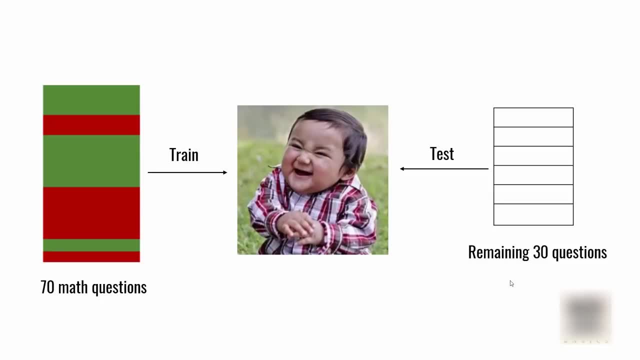 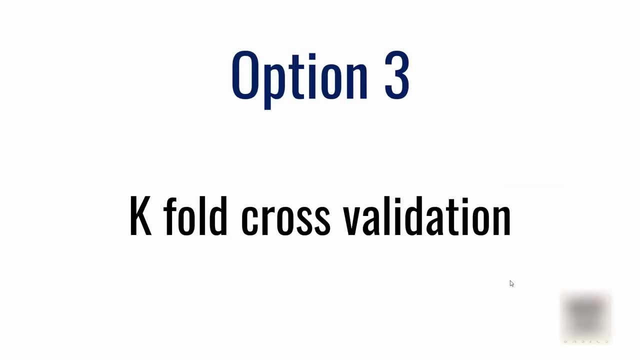 topic itself, then he might not perform well. So this, this technique is also. it kind of works okay, but it's not like very perfect. That's why we have k fold cross validation. Now, in this technique, what we do is we divide our 100 samples into folds. So I have five folds here each. 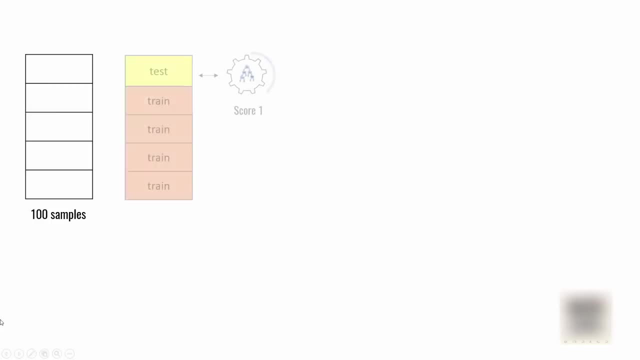 containing 20 samples, And then you run multiple iteration. In the first iteration you use fold number two to five for training the model and the first fold for testing the model and you note down the score. Second iteration: you use first fold and then three to five for training and the second one. 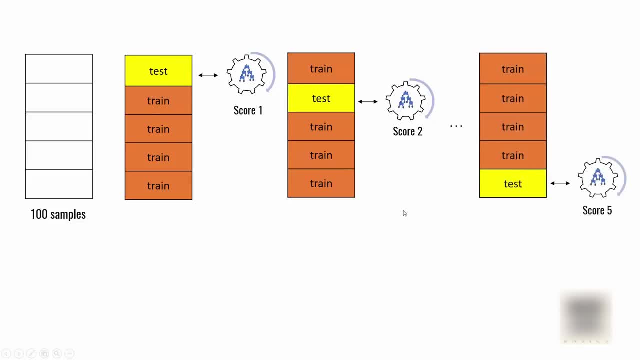 for testing, again not down the score. you repeat the process till the last fold, where you use fold number five for testing and remaining for training, And then, once you have every discourse, you just average them out. This technique is very, very good because you are giving variety of. 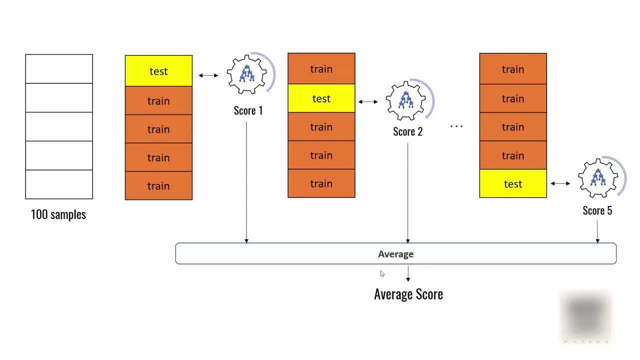 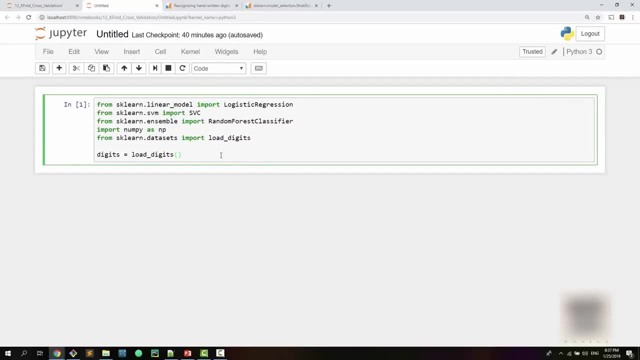 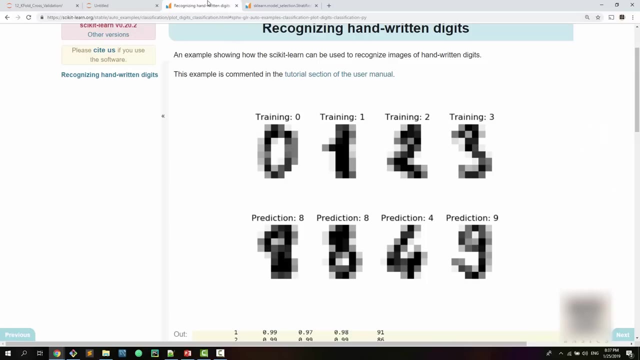 samples to your models And then you are taking individual scores and then averaging them out. Here I have imported necessary libraries that I'm going to use in this tutorial, And the purpose of this coding exercise is to classify the digits data set, which is an SQL library. you probably 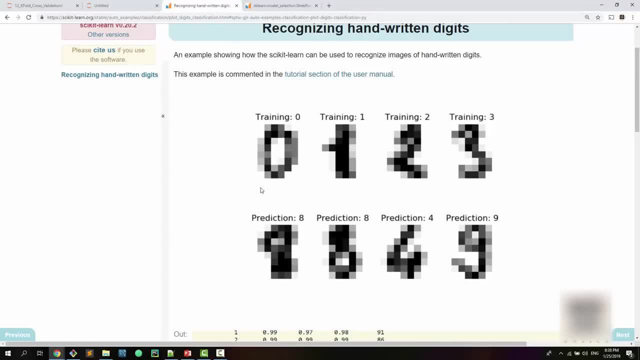 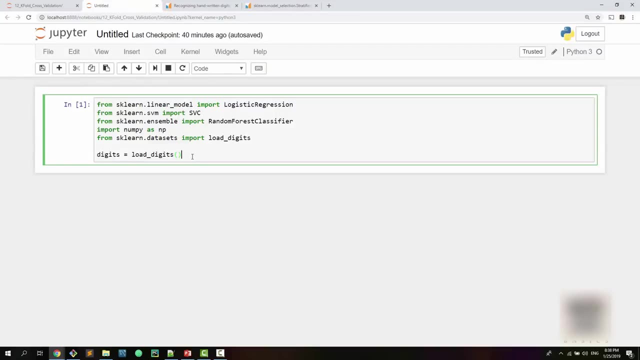 know about this. These are like handwritten characters that we can classify into one of the 10 categories, zero to nine. we will use our different algorithms, different models, and then evaluate performance of each of them using k fold cross validation. Okay, so here I imported my 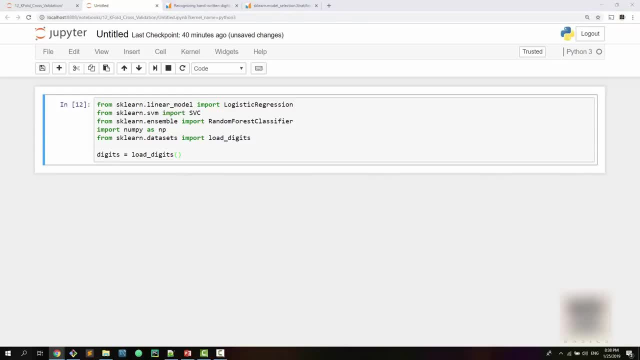 digits data set, And the first thing I'm going to do here is split that data set into training and test data set. So this is something you might be aware: that using train to split, you can split it into our training and test data sets. Okay, And once you have that, 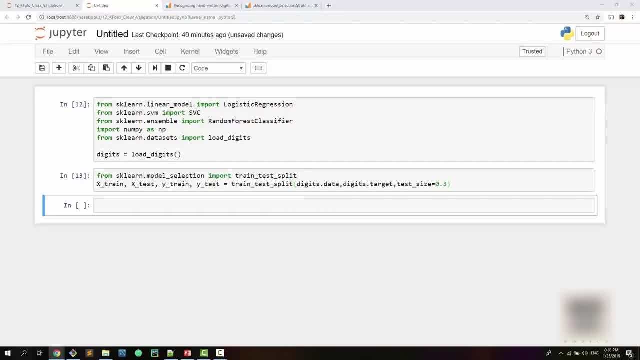 we can use a different classifier. So, for example, the first classifier I'm going to use is logistic regression And I'm going to measure the score. So here I created a logistic regression classifier. classifier is basically a machine learning model which is trying to classify your samples And I 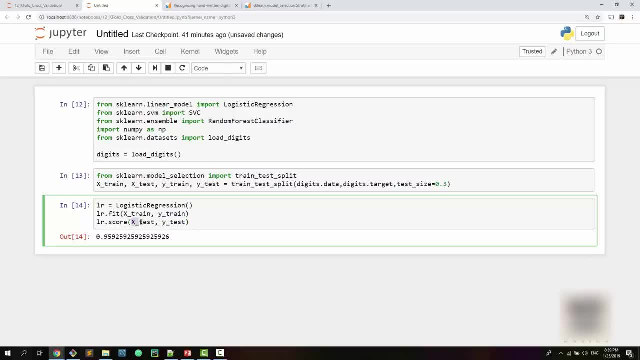 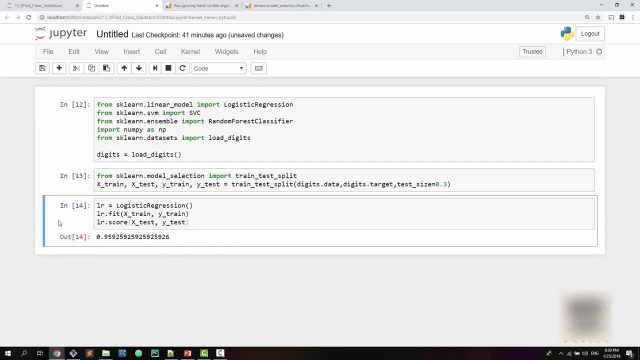 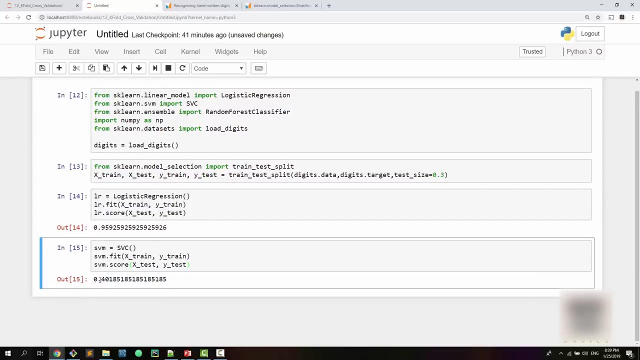 which is pretty good. Now I use logistic regression, but I have many other models as well, for example SVM. I want to try on SVM how SVM performs, So you can see SVM perform pretty poorly. it's not. the score is very low actually compared to logistic regression. I can try random forest as 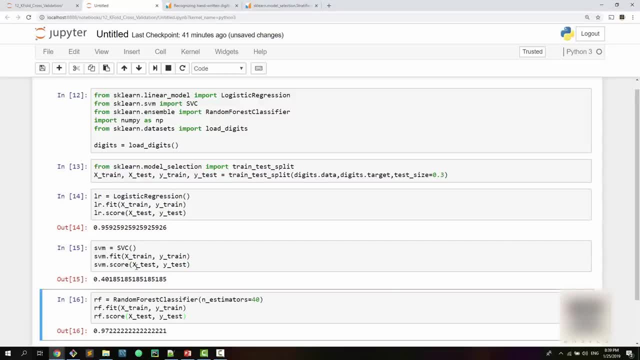 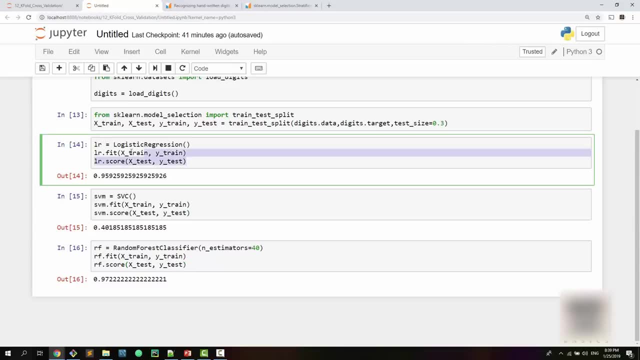 well. So in the random forest case it is performing, I think, the best. So this was a quick way of measuring the performance of these three models. Okay, so logistic regression, SVM and random forest classifier. we evaluated the performance and we found that the random forest classifier- 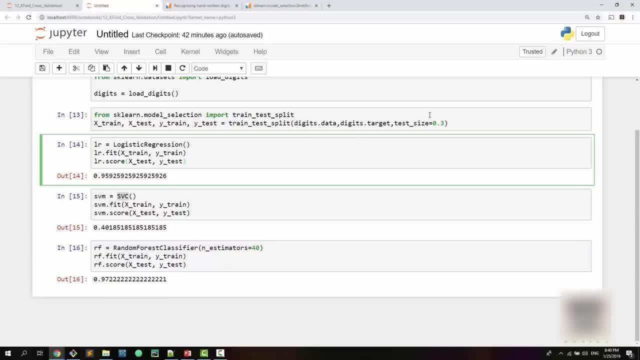 is performing the best. Now, this works in a practical situations, But what happens is the distribution of samples in an X test is not, is not uniform, right? So, for example, when I run this method one more time now, my samples change totally. So now, when I execute this code using Ctrl Enter, by the way- 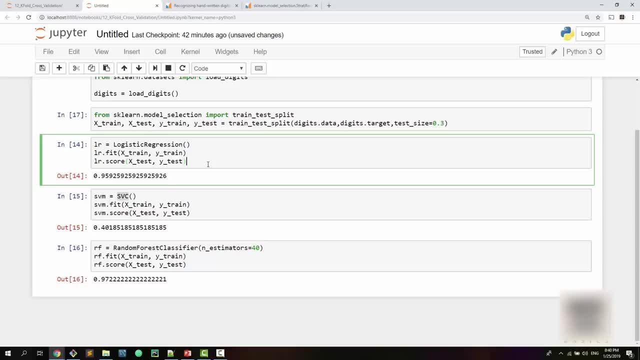 that's a shortcut in Jupyter notebook to execute yourself. you will see that the score will change. So the previous score was nine five nine. when I execute it, 953.. So it changed a little bit. Here we can see it became 0.42.. And the previous score was 99 points. So I put out the second time. 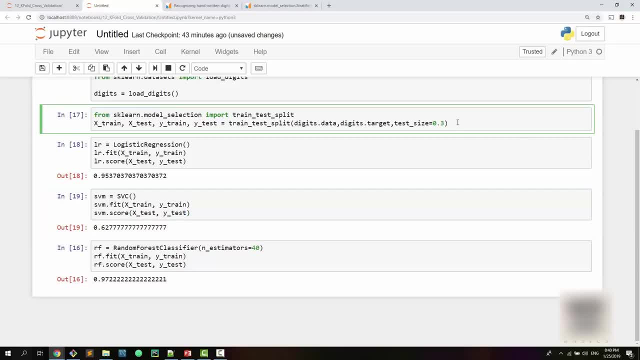 and the current score here, chicken, will be 0.20. And the previous score was conservative, so let's assume that we decide to some comes down to 0.20. And then we go back to the default test and that was zero. So I wanted to put an example, but I figured out my28, and I came. 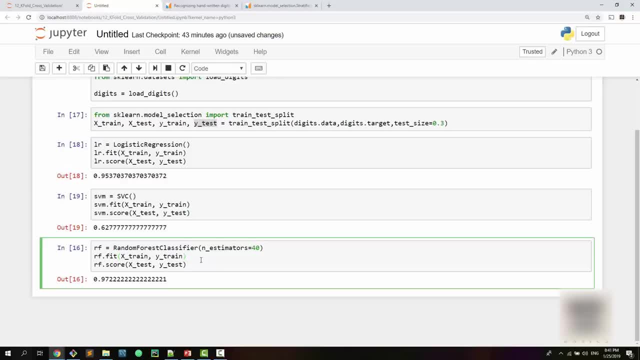 back to my final test that I already entered and that is lumped in 0.20.. Ok, so, for example, I, somewhat from on top, I considered the value of the test as 216, complement with 0.. alan the Imperial. 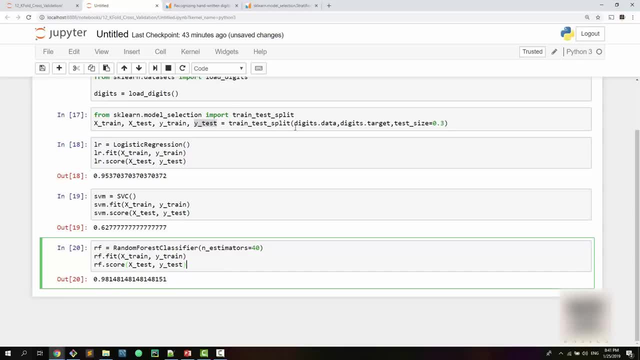 so you see the problem with train test split method, that you can't run it only one time and say that particular model is better than the other model. you have to run this multiple times, you know. so see, if i run it multiple time, every time it is changing. all right, now let's try a k. 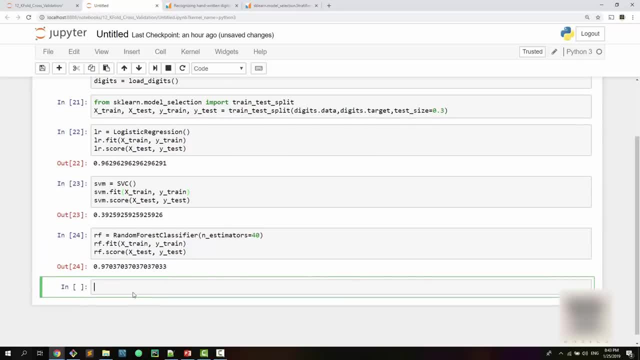 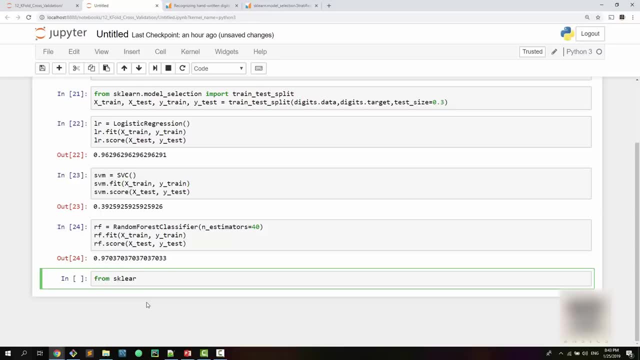 fold. so first, what i'm going to do is, uh, use k fold api to demonstrate what exactly it is doing. all right, so from escalon dot model selection you can import k fold. all right, and kf is equal to k fold. here you can specify how many folds you want to create. 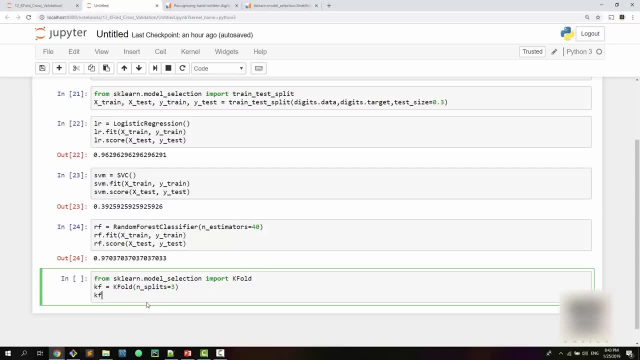 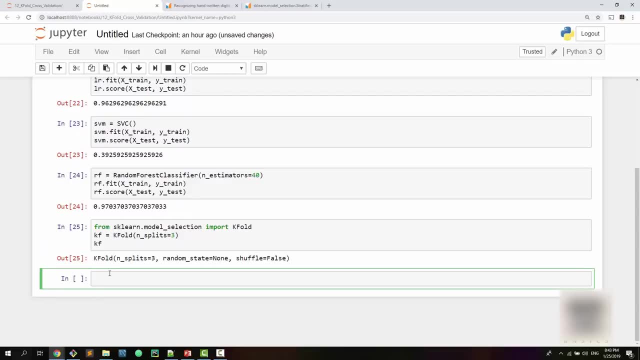 so i want to create, let's say, three folds just as an example. so here it created that. okay, and the way you use this k fold on the data set is you will say something like from train index test index in kf dot split. okay, now my k fold is ready, we know. 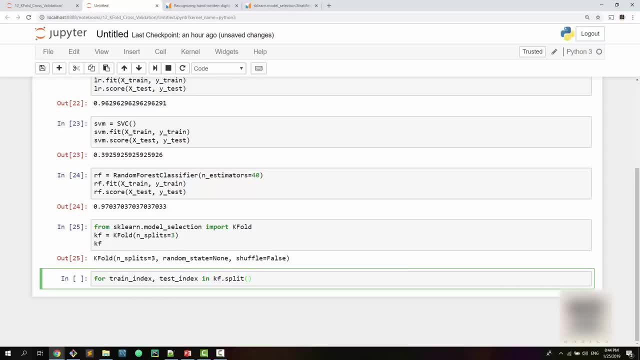 that it's gonna make three splits. so here in the argument you can supply the, the data set. all right, so let's say, for simplicity sake, i just want to supply number one to nine and then i can print train index and test index. so when i run this, what exactly is happening is: 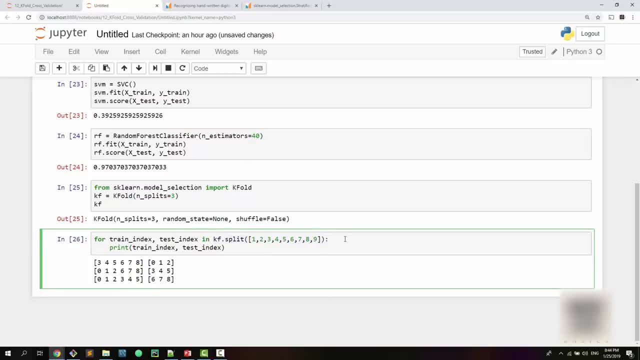 this will return an iterator, and that iterator will return train and test index for each of the four iterations. so it divided this into three folds, three each and the first iteration it used one fold for testing, which is this, and remaining two folds for training, which is this in the second. 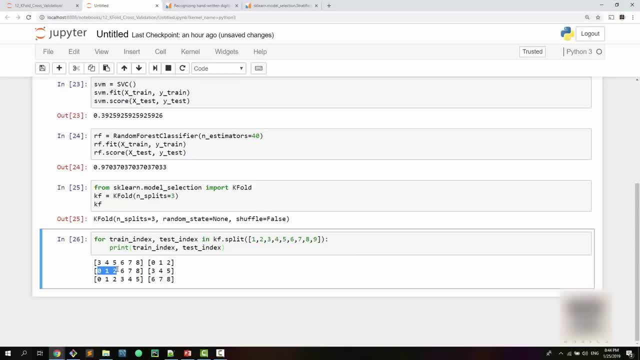 iteration. it moved this fold into training so you can see zero, one, two is in a training set, and then this fold into testing and it repeats the procedure like that so you can hear 10 folds also, and it should work accordingly. Now we are going to use k. 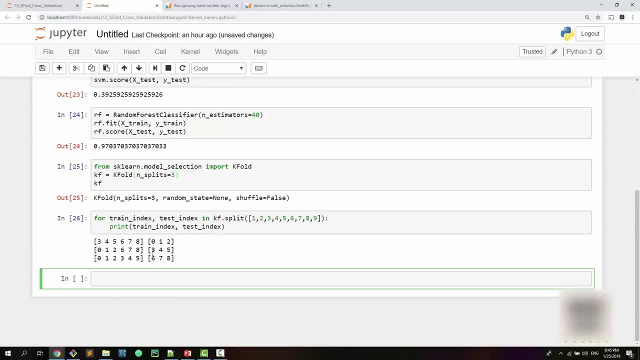 fold for our digits example. So to simplify the things, I am going to write a generic method called getScore which can take a model as an input, then xTrain, xTaste, yTrain and yTaste, and I'll tell you what's the purpose of this. 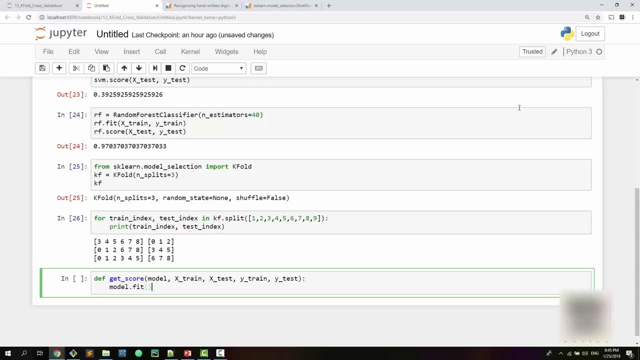 method. So this method calls modelfit, which means I want to train my model using xTrain and yTrain and once the training is done, it will return the model score using the taste sample that you are supplying as an argument to this method. Now, this method: 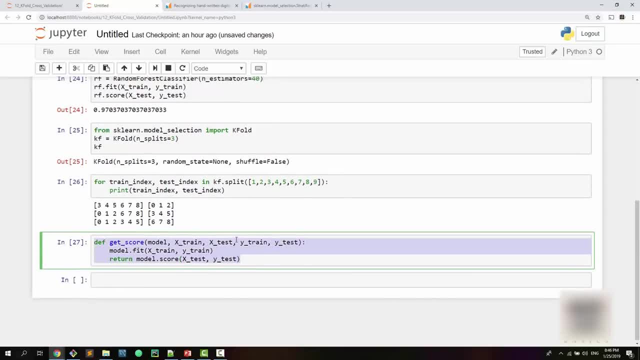 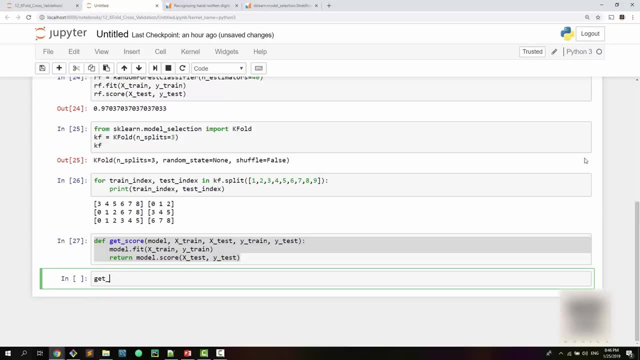 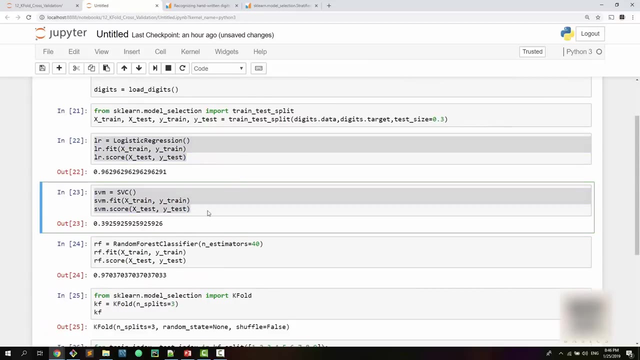 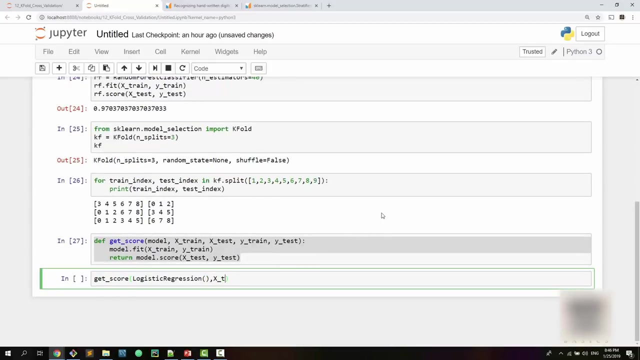 is pretty powerful. We could have used this method to measure performance of these guys as well. So, for example, let me just quickly show you If, instead of doing, you know, repeating all these three lines for each of the model, I could have just called the getScore method here on. 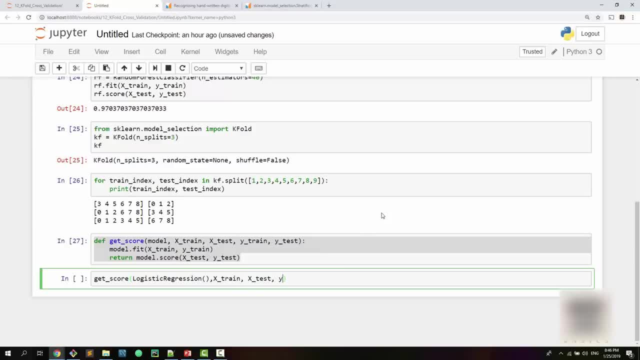 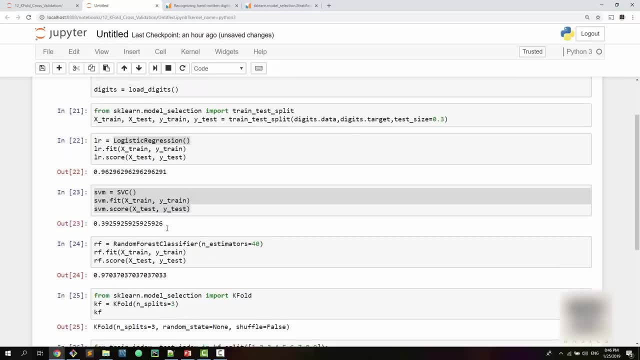 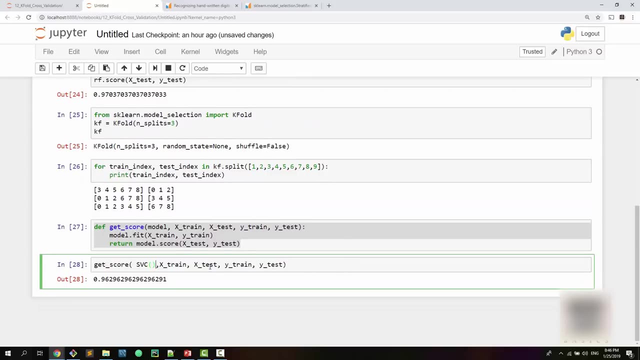 xTrain, Xtrain, Xtaste, Ytrain, Ytaste, and it should have returned me the score, alright. so same way, I could have done SVC here. so if you do SVC, it's just modularizing our core, alright. so once we have this method ready, I'm 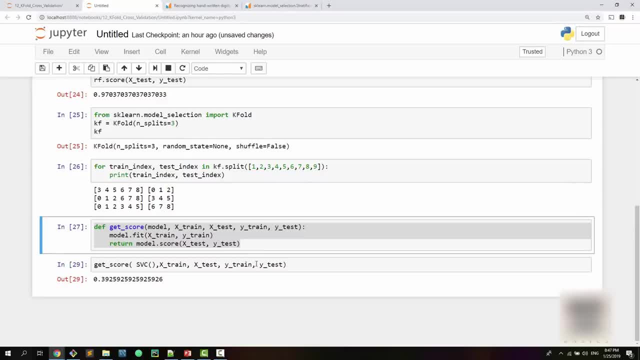 going to now use k-fold on our digits data set. so from sklearnmodelSelection, this time I am going to use stratified, stratified k-fold. so stratified k-fold is similar to k-fold, but it is little better, in a way that when you are, 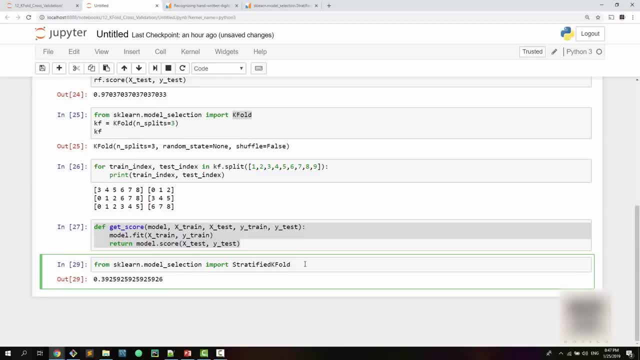 separating out your folds. it will divide your each of the classification categories uniform in a uniform way. okay, and this could be very helpful because imagine you are creating three folds, for example, our, for our iris flower data set and two flow. two folds have are two type of. 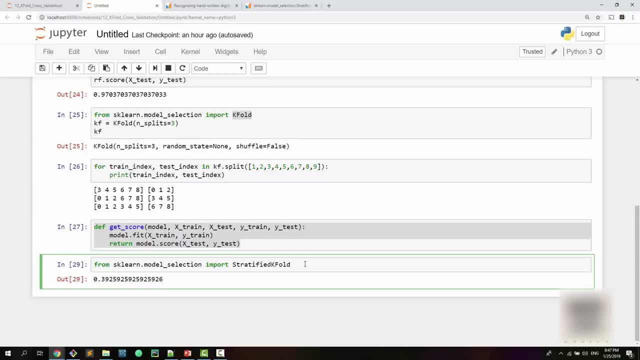 flowers and the one fold has just a very different type of flowers, then it might create problems. that's why using stratified k-fold is better. okay, so here I am going to say: my n splits is equal to 3. people usually use 10 and splits, but just to keep things simple, I am using 3 here. okay, and once you have 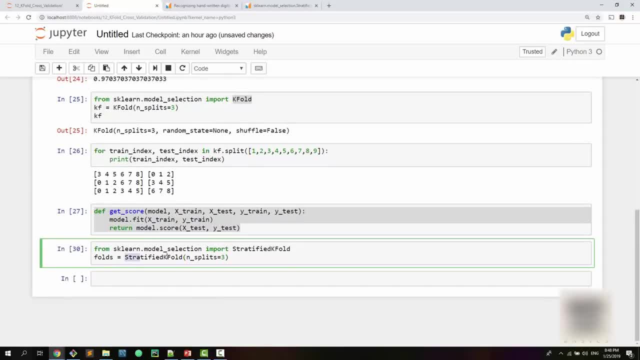 your folds ready. so this matter is exactly same as this. okay, so k-fold and stratified k-fold is same thing. so we are doing, we are repeating kind of the same thing that we did in this two lines here, but we are using now our real example of digits, data sets, and I 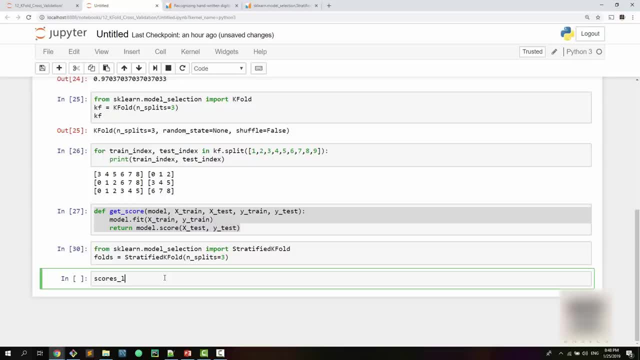 will prepare the scores array to prepare the scores of our different models. so L means the logistic regression scores and then random for a score. okay, so I need these arrays and I will tell you why I need this array. so here see, same thing. we are doing the exact same thing here. okay, but instead of this dummy data. 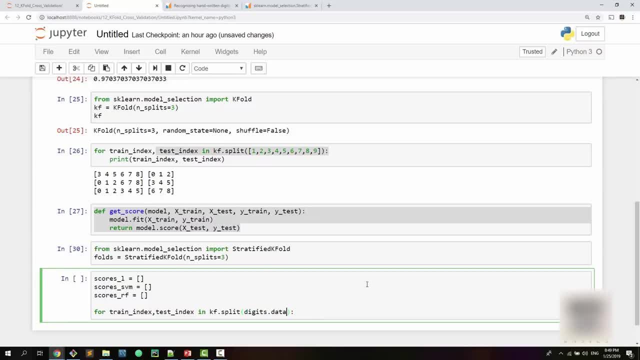 now we are using our real digits data, okay, and what will now happen is in our digits data we have train index and then again in digits data we have our test index, and these things I am going to store in x-train, x-test, y-train, y-test. okay, digits dot data. so we have train. 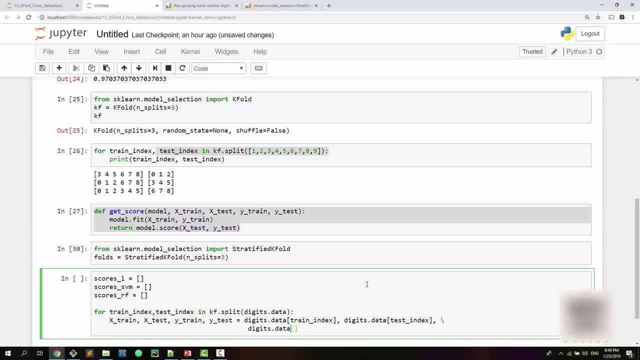 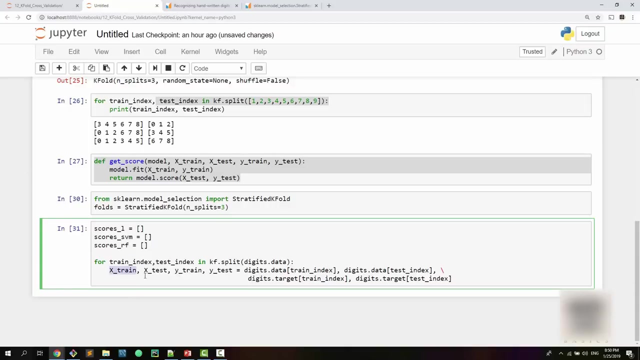 and test index. um, now i want y train, so y train is digit dot target. okay, so y train, uh train index actually. and then in the digits dot target, now i want test index. okay, if you do this, this, and if you look at the length of the each of these sets, you will realize. 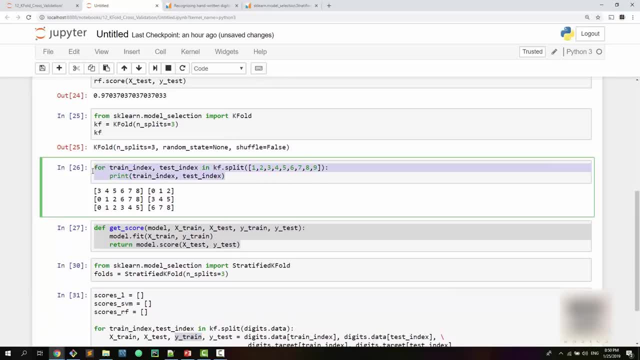 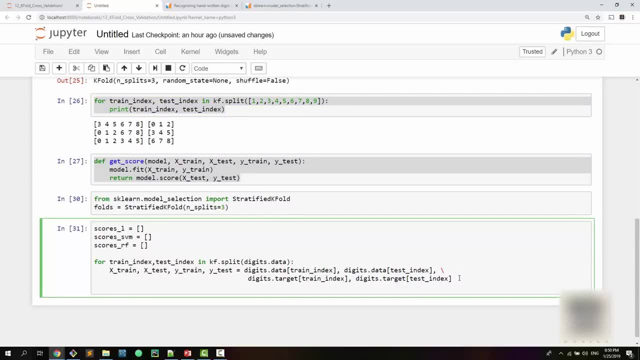 it is doing exactly same thing as it did in this cell, number 26. all, right now it's the time to measure the performance of three of our models in each iteration. so since, uh, we have three folds, this fold loop is going to repeat three times every time. we'll take this. 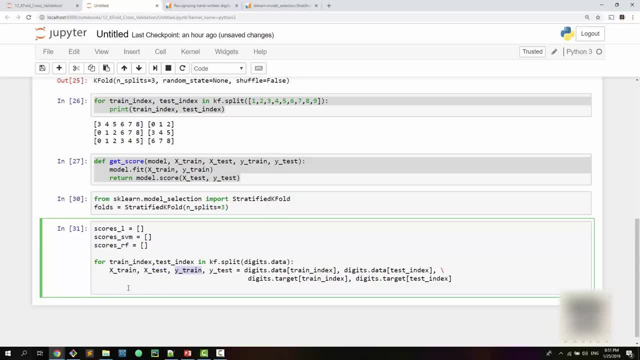 different- x test and x trains and y train and y test- and we'll measure performance of our model and then we'll append the scores in these arrays. okay, so that's what we're doing. so let's first start with get score method. so, get score method. as you know, it will 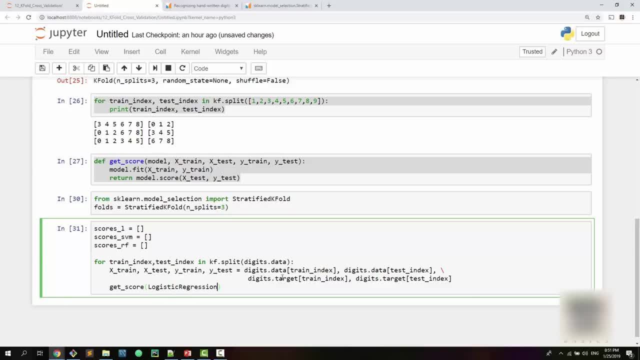 the first argument that it takes is the model. then it takes x train, x test, y train and y test. all right, let me just print this, and i can do the same thing for three different models. so the second model is svm and the third model is random forest classifier. 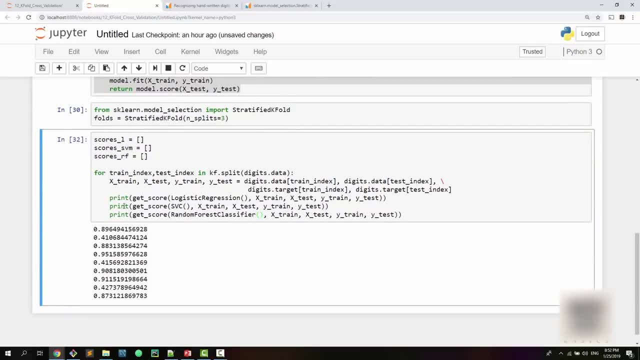 when i print the scores, it is printing the different scores. okay. so first iteration, these are the three model performance. second iteration and third iteration. now, instead of just printing, why don't we append the same score here? so instead of printing, i'll say: append that exact same score. 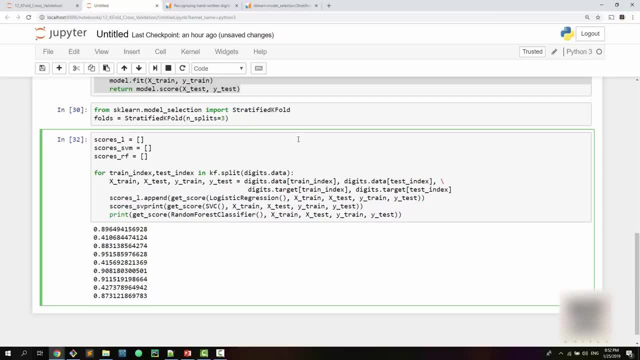 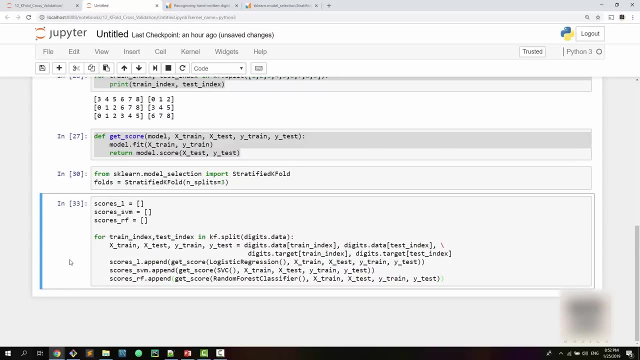 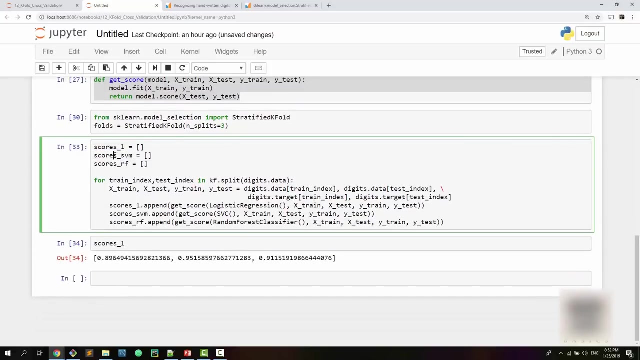 here. now let's sayации Bugün. so'm gonna print this into here in light of the last event. all right, so let me just piece it up again again. so now what we need to do is just copy this, these two elements, and we will be printing them. 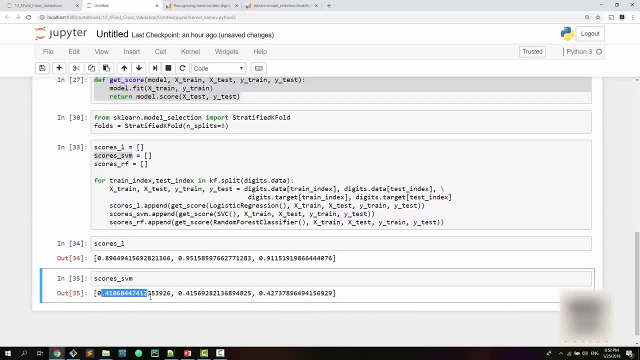 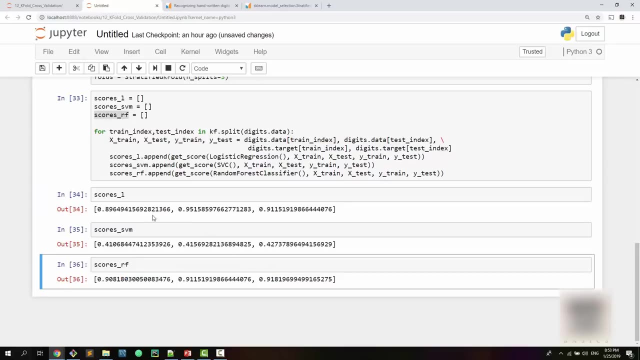 ity, we'll print them, write timesicos so saying diferencia, find intellect chart, seminal code and we're going to print this asС 하. not that great and we have seen the same behavior before. all right, so logistic regression and random, for us looks to be performing similar almost right on one. 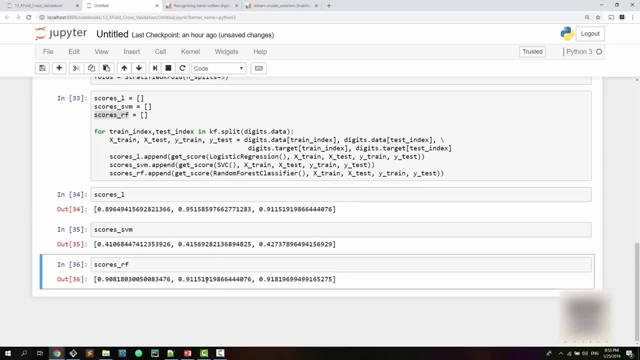 instance, this guy perform little better. but what you can do is now you can take the average of these three scores and you can determine what is the best model for a given problem. here it looks like based on this, it looks like our logistic regression model might perform the best one optimization I can think of doing. 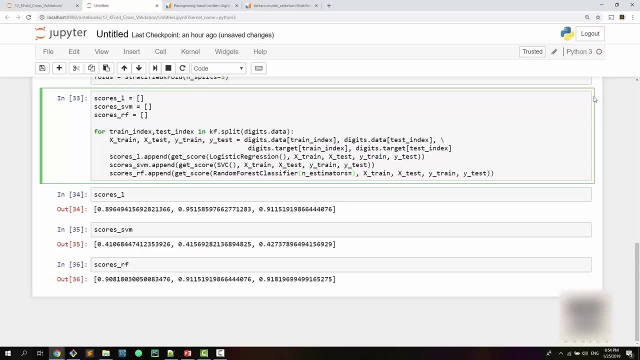 here is increased number of trees in my random forest classifier. so if I increase the trees to 40, let's see how it performs. all right, I increase the trees to 40 and my scores are ready. so now I will once again evaluate this course. nice, so you can see. now random forest seems to be doing better because in 95 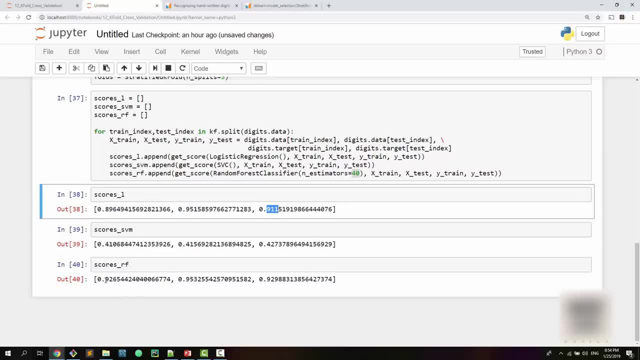 score matches here, but here is 89, 91 and here is 92 and 92. so now, after I did little tweaking, a parameter tuning in my random forest classifier, my scores improved. now this code looks little messy because we have to deal with so many indexes, but luckily 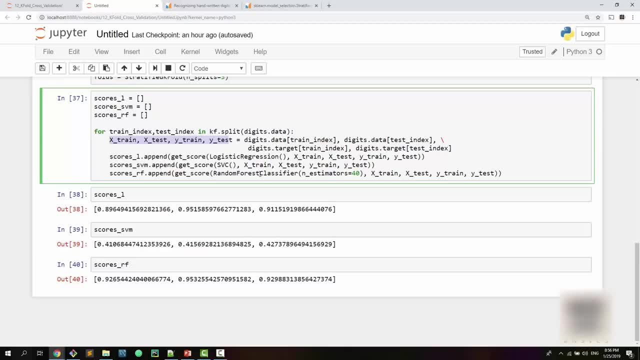 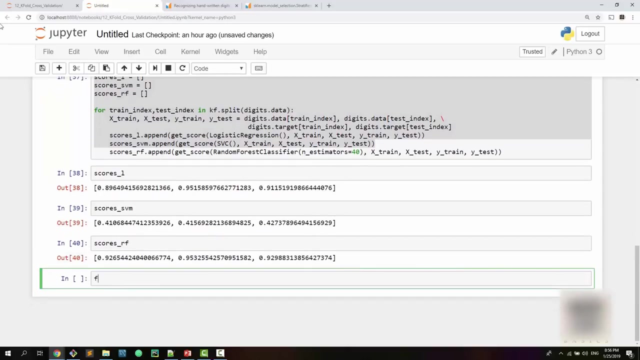 things we have solved totally vote as well. we didn't solve all of them, but we'll give some extra time to provide some 1930 points. we can tweak them if needed. but if you wanted them to have some more value later, we can do little tweaks in the 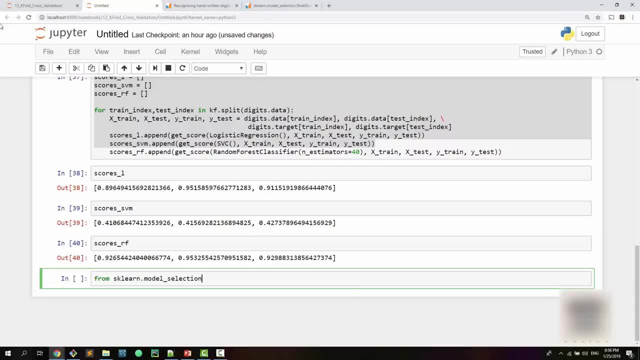 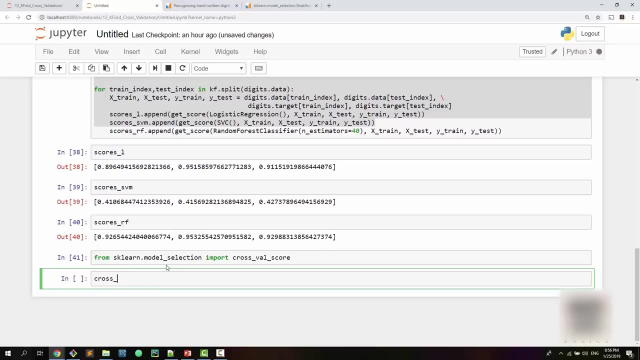 whole table soon. so now we are satisfied. you know watching all of these ones. actually, every one of you can import the method from sklearn model selection- it's called cross val score, okay, and once the method is imported, you can call this method with first argument is your classifier. 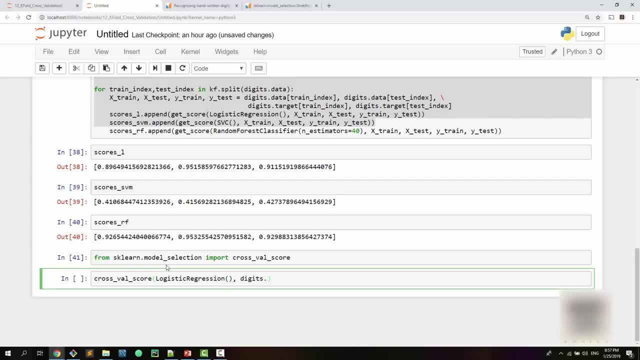 the second argument is your x, which is digits dot data. the third argument is your y, which is digits dot target. so if you do shift tab to look at the, the documentation, it says estimator, which is a model. the second argument is your x and third argument is y. so that's what we did and 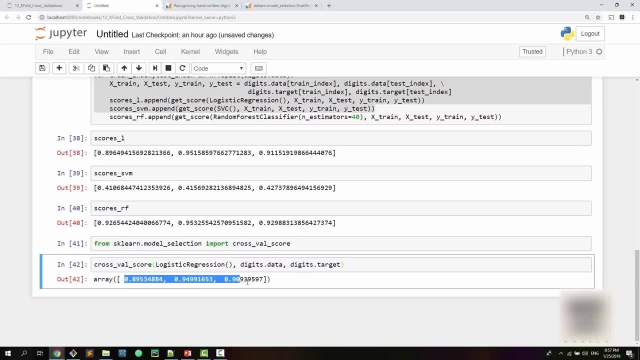 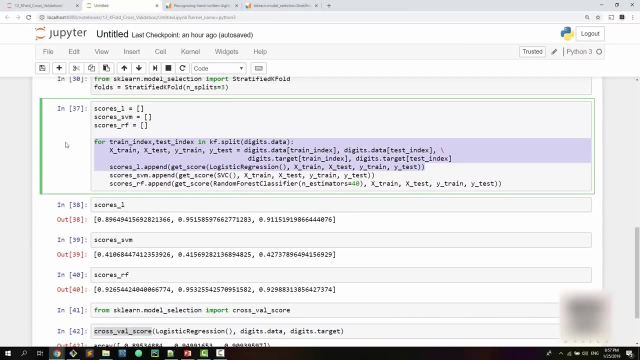 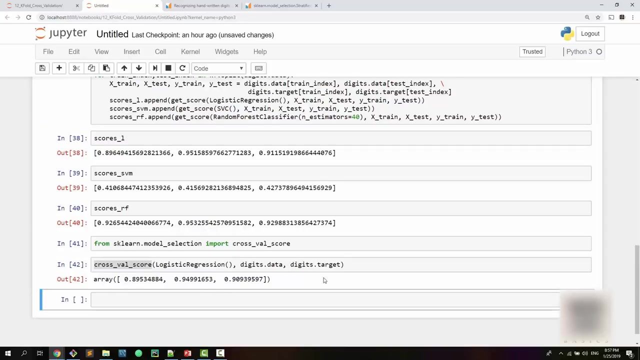 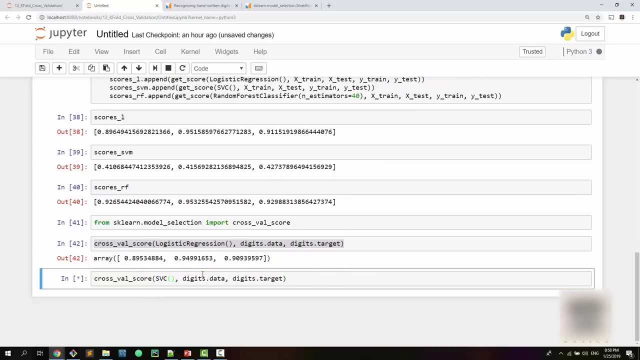 when you execute this line, this is showing you the similar score, basically right, so that score is being shown here. so internally, this method did the same thing as this for look. basically it created folds and it measured the performance and it prepared this course array. okay, i will now call the same method on my svm classifier and see how that goes. 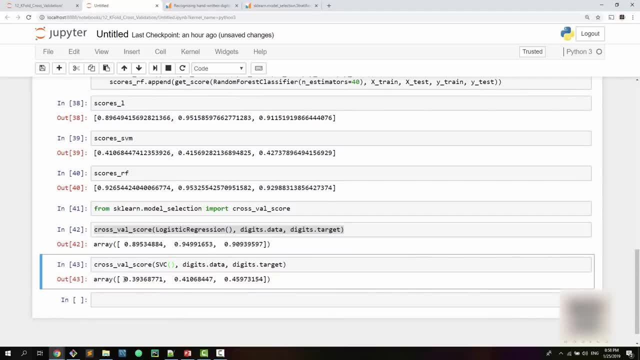 again. svm didn't perform again. svm didn't perform again. svm didn't perform really well. my accuracy is 39 percent 41, really well. my accuracy is 39 percent: 41, really well. my accuracy is 39 percent: 41 person and so on, versus here: 89. 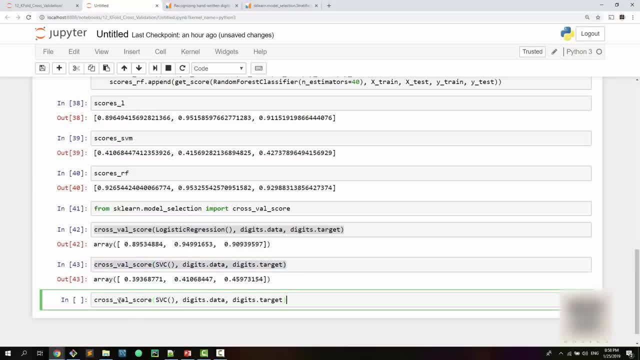 person and so on. versus here 89 person and so on. versus here 89, 94 person, it's much better, and in the 94 person it's much better, and in the 94 person it's much better. and in the third case i'll just copy paste. 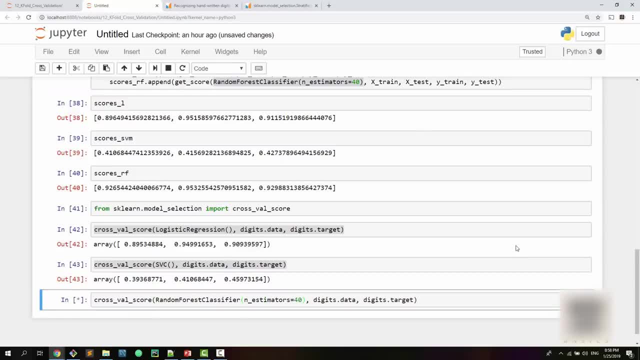 third case. i'll just copy paste third case. i'll just copy paste this code here. so see, all you have to do is just call. so see, all you have to do is just call. so see, all you have to do is just call one line. man, it's machine learning is. 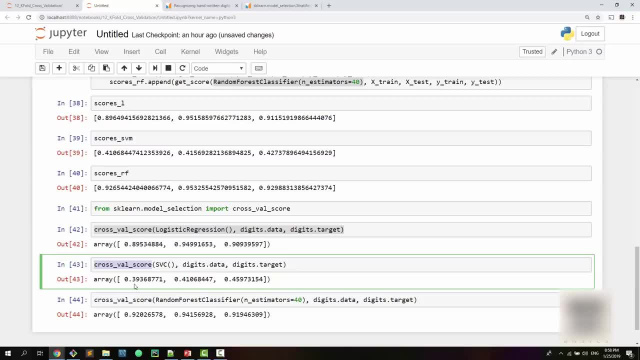 one line man. it's machine learning is one line man. it's machine learning is not hard. if you know the internals of not hard, if you know the internals of not hard, if you know the internals of these libraries, then all you need to do these libraries, then all you need to do. 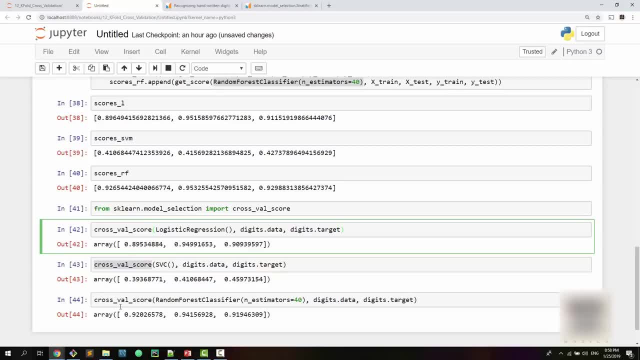 these libraries, then all you need to do is just just call one single method and is just just call one single method and is just just call one single method and say it's measuring the performance. now say it's measuring the performance. now say it's measuring the performance, now we. 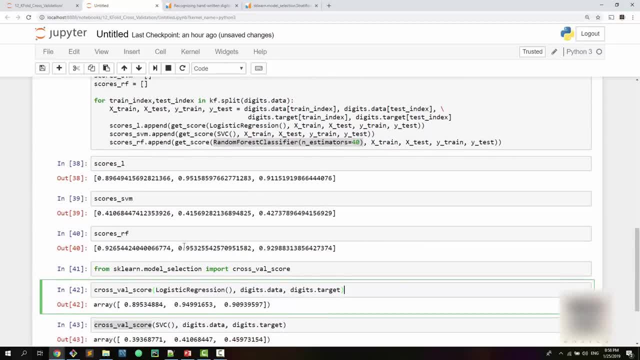 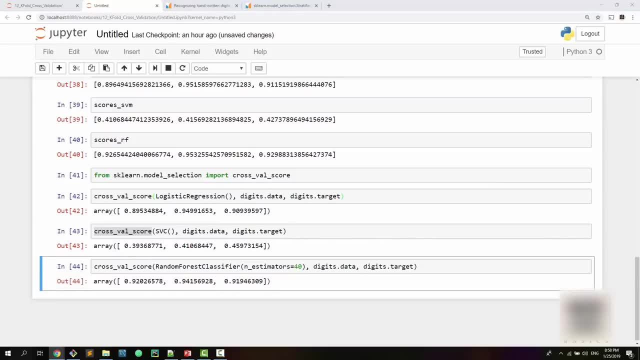 we. we compared different classifiers. you can compared different classifiers. you can compared different classifiers. you can compare same classifier with different. compare same classifier with different. compare same classifier with different parameters, parameters, parameters- this is called parameter tuning. for this is called parameter tuning, for this is called parameter tuning. for example, we have random forest classifier. 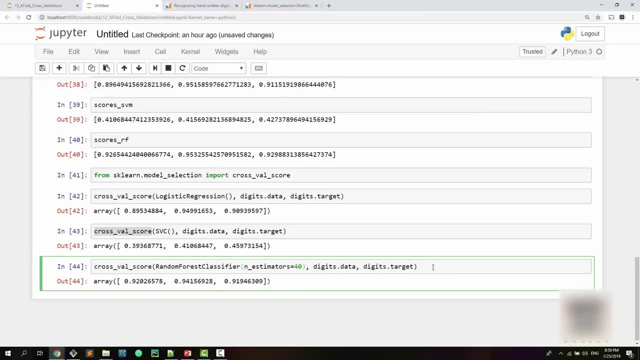 example, we have random forest classifier. example. we have random forest classifier right here and random forest right here and random forest right here and random forest classifier. we ran with classifier, we ran with classifier. we ran with 40 trees. we can actually 40 trees. we can actually. 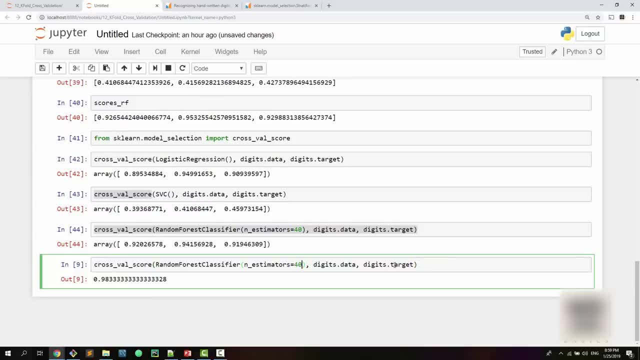 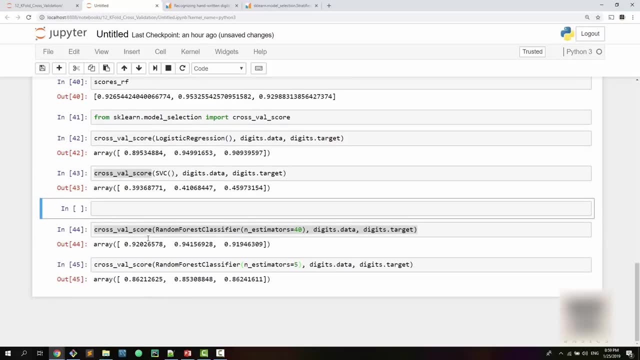 40 trees. we can actually uh, run the same classifier with, let's say, run the same classifier with, let's say, run the same classifier with, let's say, five trees, and get the score okay. so you see this and get the score okay. so you see this. 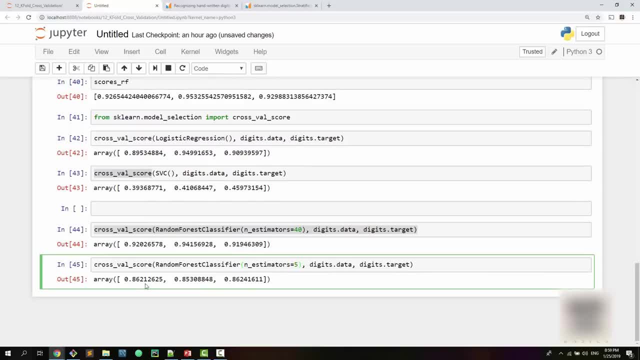 and get the score okay. so you see, this is 40 classifier. this is the score with is 40 classifier. this is the score with is 40 classifier. this is the score with five classifier. we say the score went five classifier. we say the score went five classifier. we say the score went down a little bit. 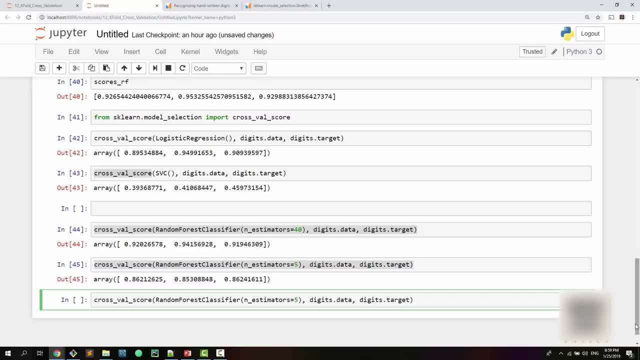 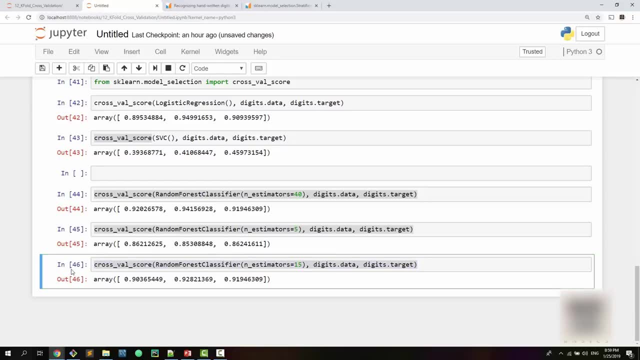 down a little bit, down a little bit. let me try: 15, for example, 15, for example, 15, for example, and the score and the score, and the score went and the score went and little bit up and little bit up and little bit up, okay, okay. 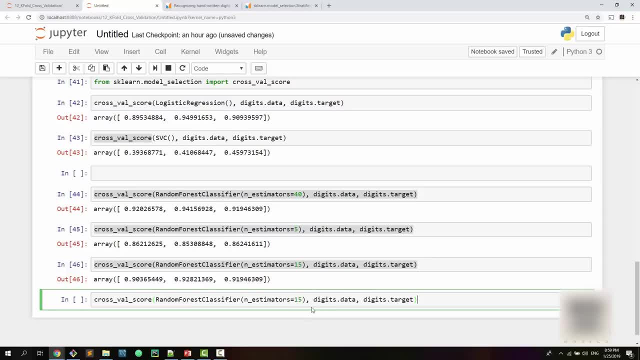 okay. so looks like, as i increase my trees, my so looks like. as i increase my trees, my so looks like, as i increase my trees, my score is increasing. score is increasing. score is increasing. so how about if i make my trees to be 50? so how about if i make my trees to be 50? 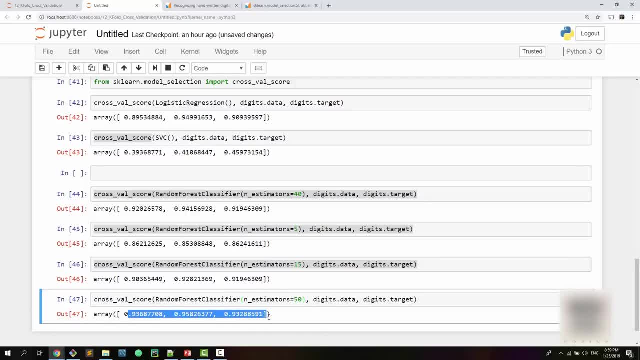 so how about if i make my trees to be 50, so with 50, so with 50, so with 50. it increased even further, it increased even further. it increased even further. 60, 60, 60, okay, 60, okay, 60, okay, 60. i think 50 was better than 60. so so, 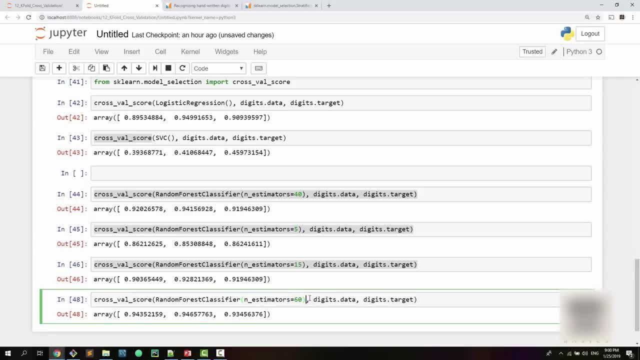 i think 50 was better than 60. so so i think 50 was better than 60.. so so this way, this way, this way you can take, you can take, you can take a model, a model, a model, and then you can do parameter tuning. so 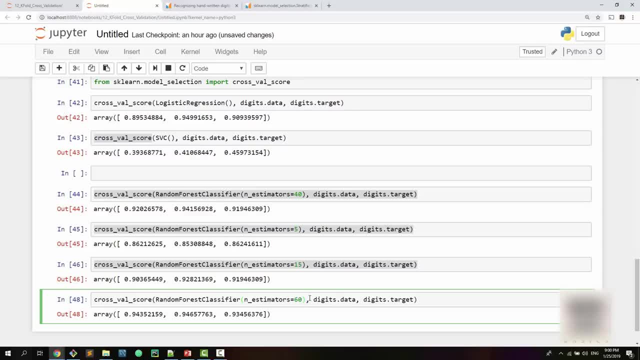 and then you can do parameter tuning. so, and then you can do parameter tuning, so you're using the same algorithm. you're using the same algorithm. you're using the same algorithm. basically here, random forest classifier. basically here, random forest classifier. basically here, random forest classifier. but then you are tuning the parameters. 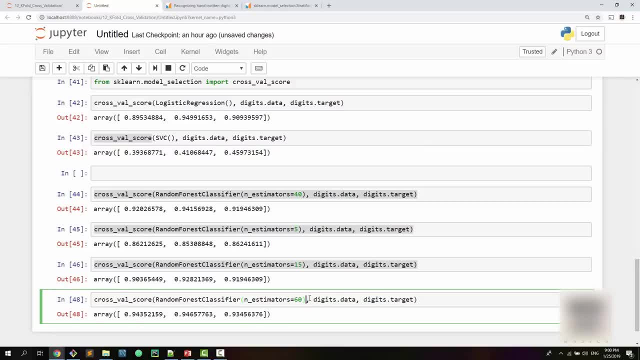 but then you are tuning the parameters, but then you are tuning the parameters and trying to gauge, and trying to gauge, and trying to gauge which one delivers the best performance, which one delivers the best performance, which one delivers the best performance. so you can see that cross validation. 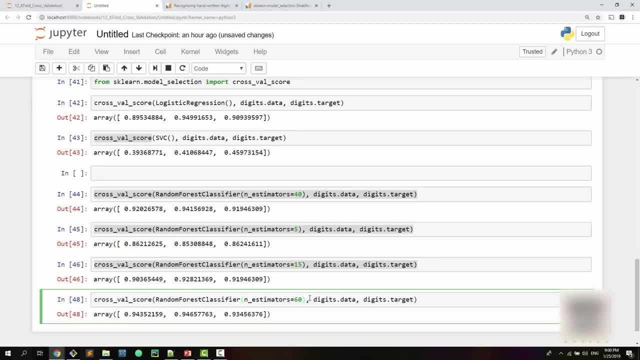 so you can see that cross validation, so you can see that cross validation technique is pretty useful. it not only technique is pretty useful. it not only technique is pretty useful. it not only allows you to, allows you to, allows you to compare different algorithms, but the. compare different algorithms, but the. 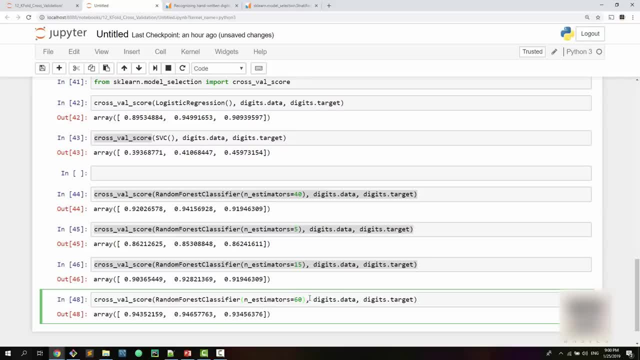 compare different algorithms, but the same algorithm with different parameters. same algorithm with different parameters. same algorithm with different parameters. how it would behave for your given. how it would behave for your given. how it would behave for your given problem. it can tell you that. okay, so problem. it can tell you that. okay, so. 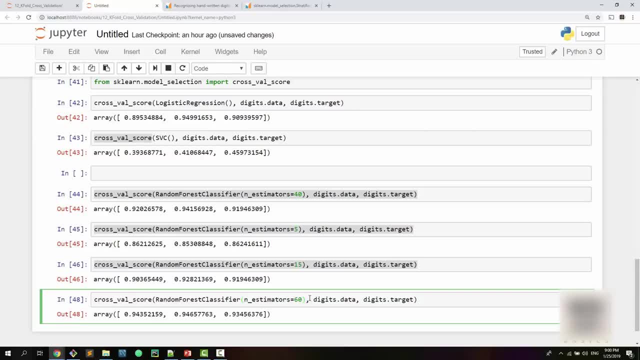 problem, it can tell you that. okay. so machine learning is not like a. machine learning is not like a machine learning is not like a scientific equation. where scientific equation? where scientific equation? where, for a given problem, you use this model? for a given problem, you use this model. 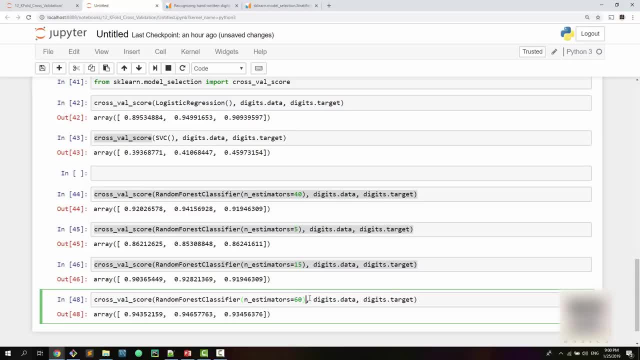 for a given problem. you use this model versus that model. is something versus that model, is something versus that model, is something a little bit like trial and error based. a little bit like trial and error based. a little bit like trial and error based where, where, where, for your given problem and given data. 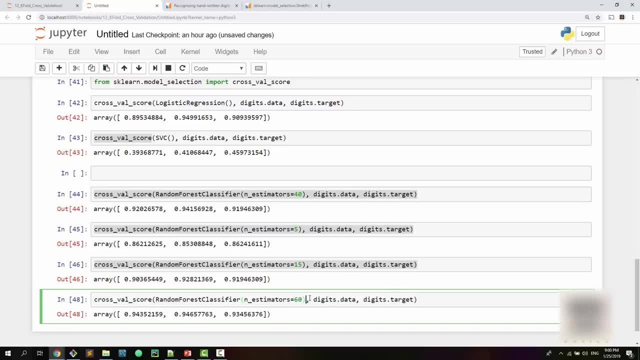 for your given problem and given data. for your given problem and given data, set, you need to try various models with set. you need to try various models with set. you need to try various models with various parameters, and then various parameters, and then various parameters, and then figure out which one is the best for. 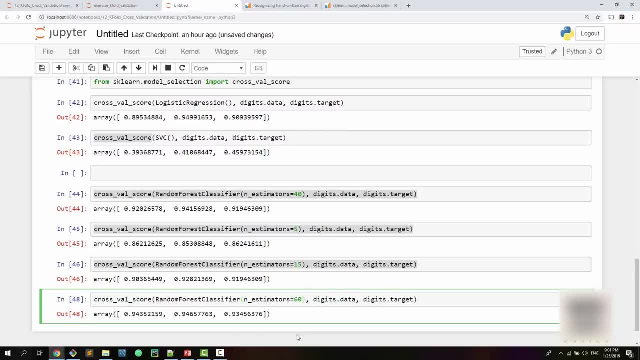 figure out which one is the best for, figure out which one is the best for your use case. all right now. now comes your use case, all right now. now comes your use case, all right now. now comes the most interesting part, which is the. the most interesting part, which is the. 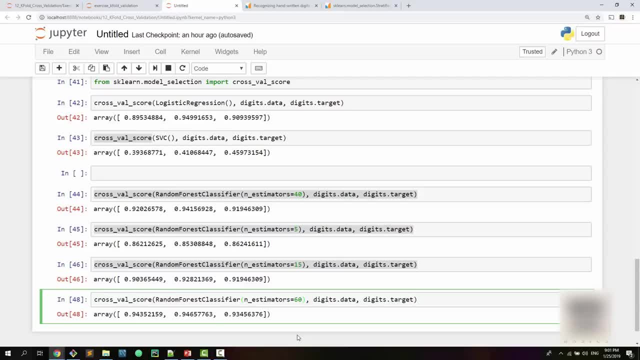 the most interesting part, which is the exercise. so what we want to do this exercise? so what we want to do this exercise. so what we want to do this tutorial is: take the iris flower data tutorial is take the iris flower data tutorial is take the iris flower data set and use different classifier: random. 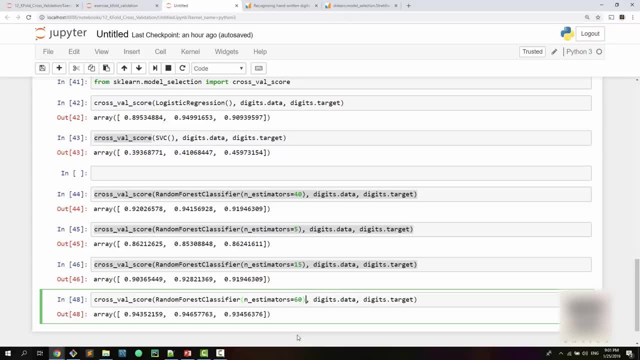 set and use different classifier: random set and use different classifier: random forest decision tree- svm. and logistic forest decision tree- svm. and logistic forest decision tree- svm. and logistic regression, regression, regression and use crosswell score method to measure and use crosswell score method to measure and use crosswell score method to measure the performance of the base classifier. 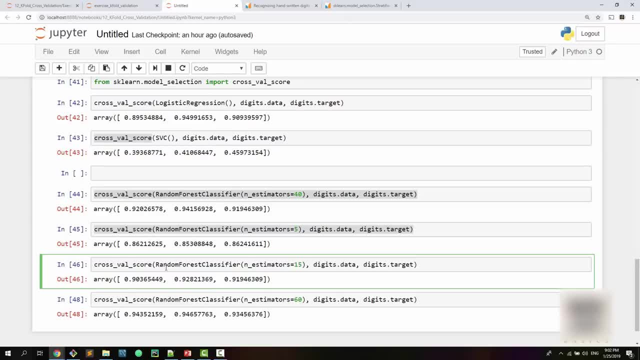 the performance of the base classifier. the performance of the base classifier. so, for example, if i'm a teacher and i'm so, for example, if i'm a teacher and i'm so, for example, if i'm a teacher and i'm telling you to, telling you to. 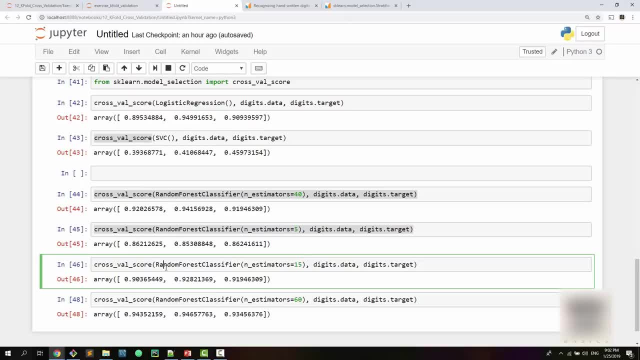 telling you to solve the classification problem of iris. solve the classification problem of iris. solve the classification problem of iris. flower: which model will you use so you'll flower? which model will you use so you'll flower? which model will you use so you'll use? use, use crosswell score with these four different. 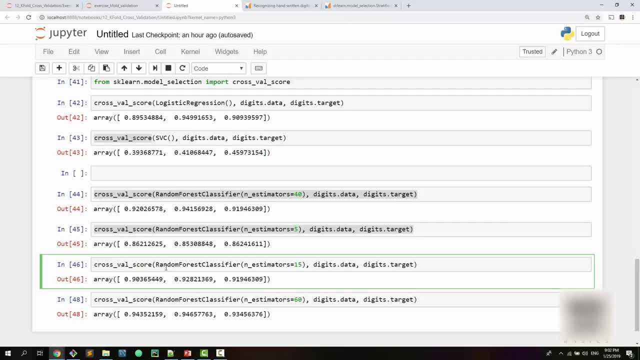 crosswell score with these four different crosswell score with these four different models, and you will tell me models and you will tell me models and you will tell me which model performs the best, all right. which model performs the best? all right. which model performs the best? all right, that's all i had for this tutorial. i. 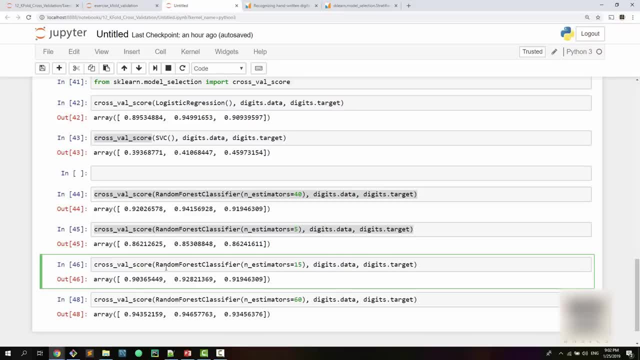 that's all i had for this tutorial. i that's all i had for this tutorial. i have a link, have a link, have a link of jupiter notebook used in this tutorial, of jupiter notebook used in this tutorial. of jupiter notebook used in this tutorial, as well as exercise. 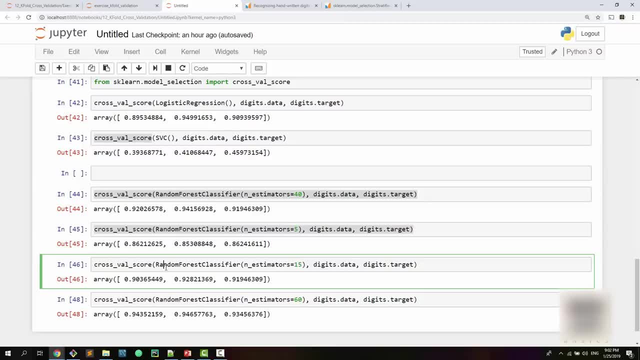 as well as exercise, as well as exercise. uh in the description down below. uh in the description down below. uh in the description down below. in the video description section. in the video description section, in the video description section. and stay tuned, i'll be back with the next.